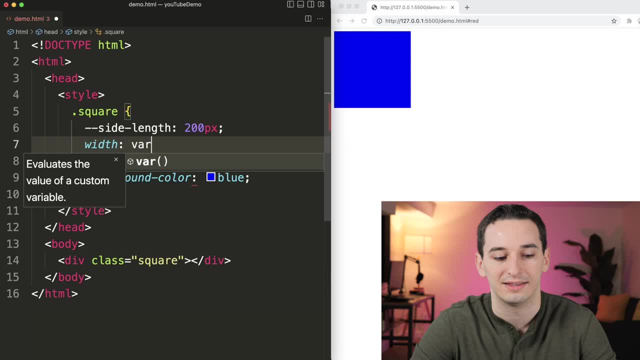 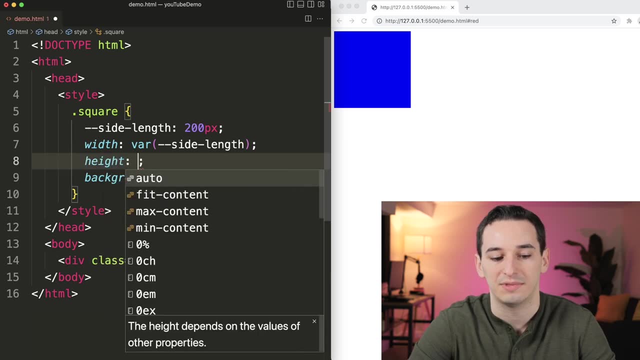 in our CSS code. we can use that side length So we can say: this is a variable, So we have this variable function And then we pass in that name And that's going to be our width, And we can do the same thing for height. So we can say: the variable of side length, save this, and it still 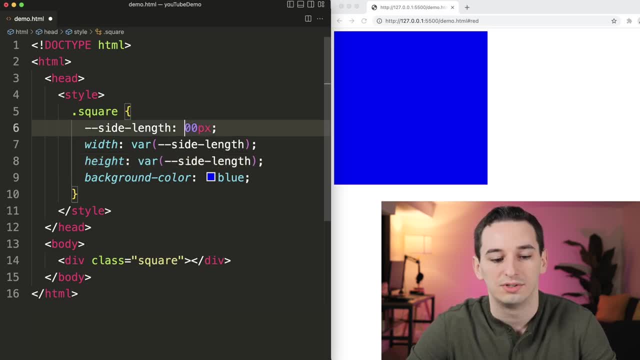 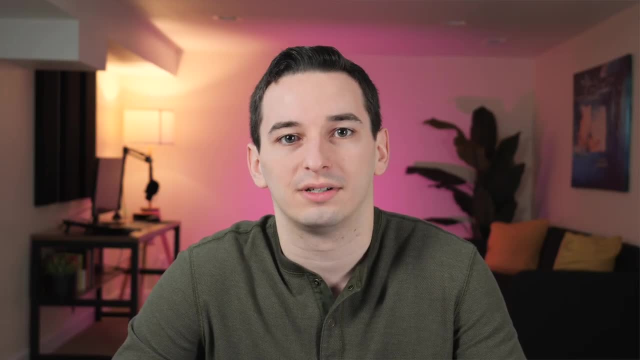 works. And then if I was to change this value to say 400 or maybe 500 pixels, it is going to keep updating the width and the height, And these variables, or custom properties, as they are technically called, can be super useful for lots of things. So, for example, in most of my projects. 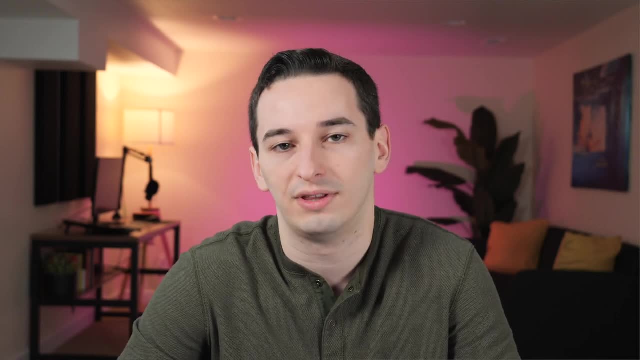 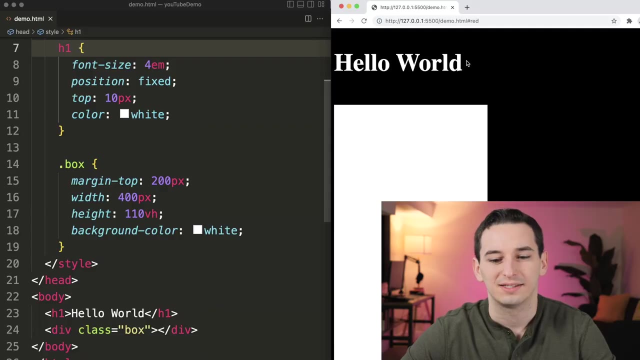 I create these global custom properties that I can use through the entire CSS files for things like the colors of the website. to make sure I'm being consistent Here, I have this H1 that says hello world And it's white And it's over this white box, But the H1 has position fixed. So if 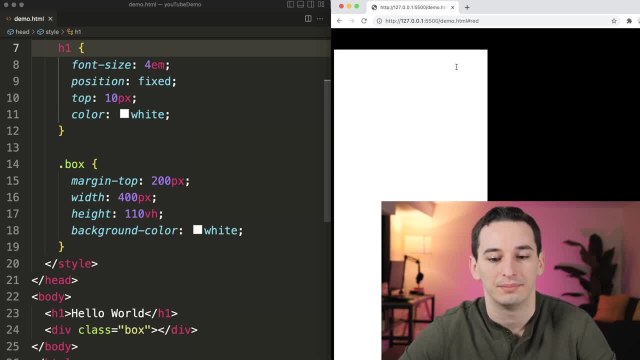 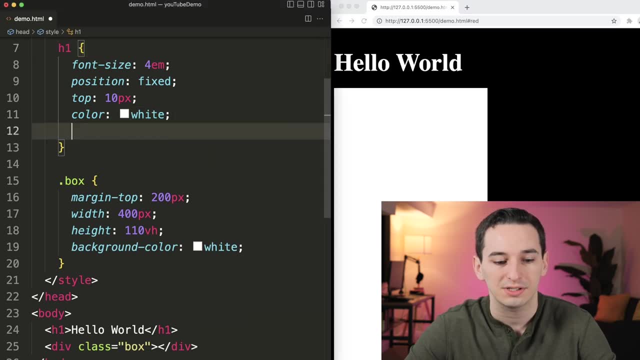 scroll, it stays in the same spot, But we can see it gets covered by the white box If I scroll too far. So how can we solve this? How can we make sure that we can always see this text? Well, for this we can use something known as a mix blend mode, which allows you to say: 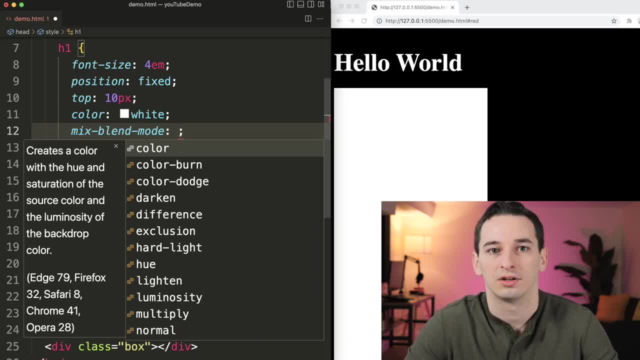 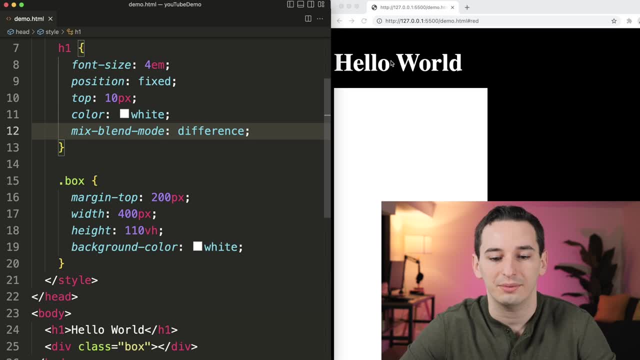 how is this element going to be affected by the color of the background? So, for example, we can set this to be difference, which is basically going to subtract the two colors from each other. It's not when I save this, this stays as white, But when we scroll over the white, 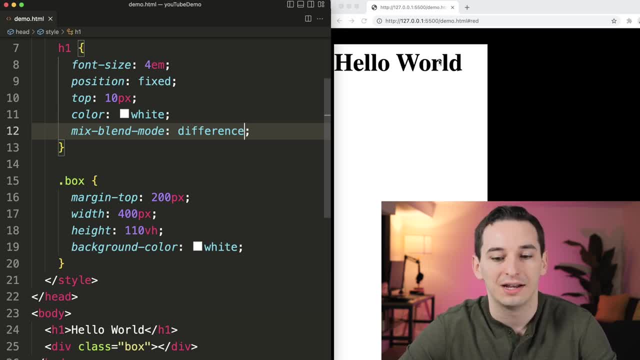 box. it changes to black to be the opposite color, And we can even see if it's half color or half color, And we can even see if it's half color or half color. And we can even see if the top half stays as white and the bottom half is going to be black. And now there are a bunch. 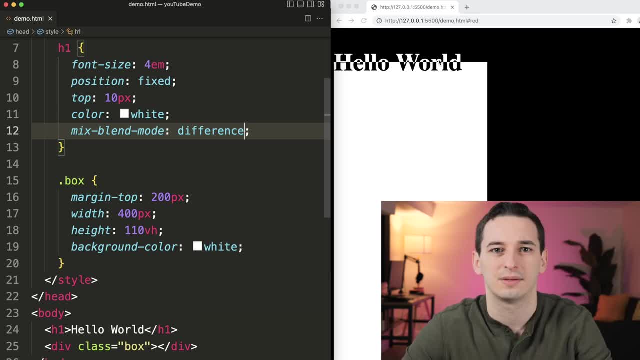 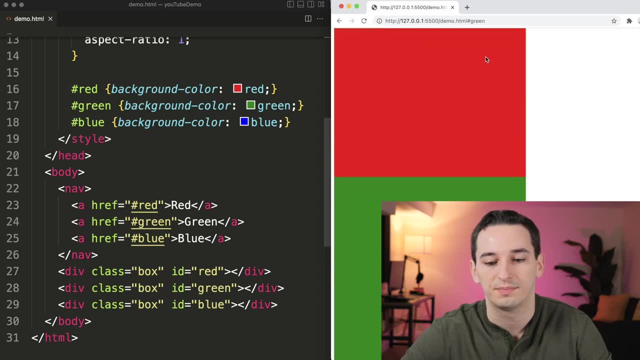 of different mix blend modes, So I will leave a link down in the description If you're interested in learning more about the different options here. we have three boxes- red, green and blue- and we have links to all of those boxes, which is done using these anchor tags in the HTML. 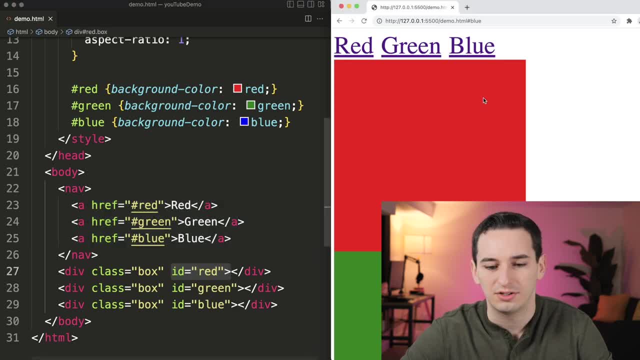 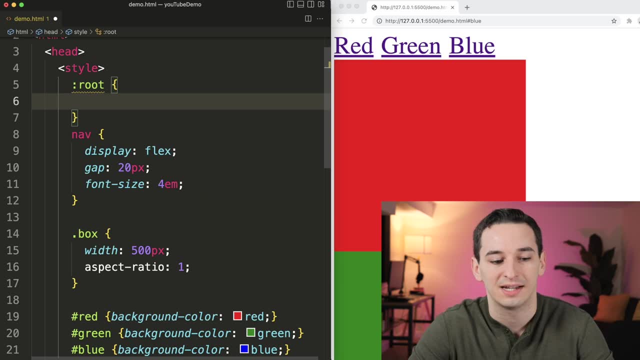 which link to these different IDs. But what if we wanted to more smoothly scroll? Well, for that we can add smooth scroll. So we can say, on the root selector, which is going to affect the entire page, we can say that we want to have smooth scroll. So this: